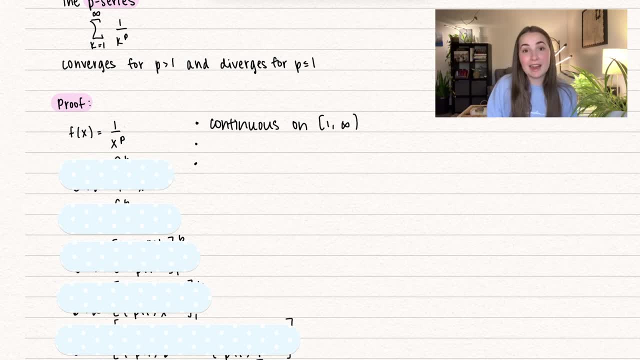 it's not in the domain. So we have that it's continuous. We also need to have that it's positive. Well, we're only plugging in positive numbers and no matter what power it is, a positive number to any power is always positive. So we have that it's continuous. We have that it's positive. 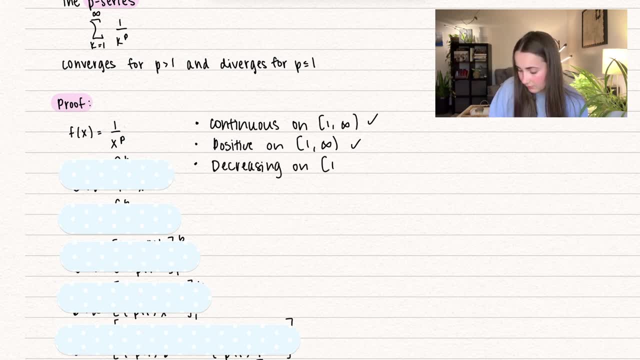 We also need to have that. it's decreasing. We know that this is going to be decreasing because, as x gets larger and larger, 1 over that larger number becomes smaller and smaller. right Like if we had 1 over x squared, we would have 1 over 1 squared, which is just 1.. We'd have 1 over 2. 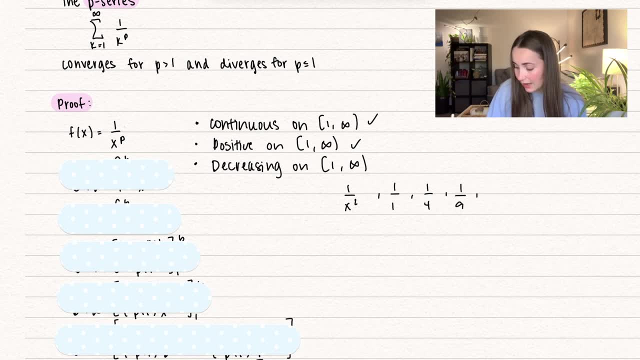 squared, which is 1. fourth, 1 over 3. squared, which is 1. ninth right, And we would just be getting smaller and smaller, No matter what the exponent is. that's going to be the same pattern, right? So, since all of these three conditions are met, we can go ahead and use the integral test. 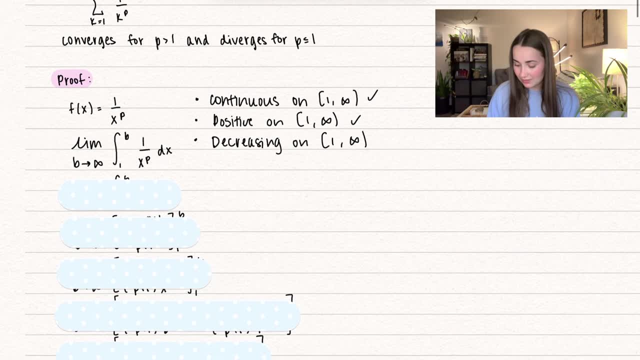 So what we're going to do is set up our integral. We're going to take the limit as b approaches. our lower limit is 1, our upper limit is b, and then we have 1 over x to the p dx. So let's go. 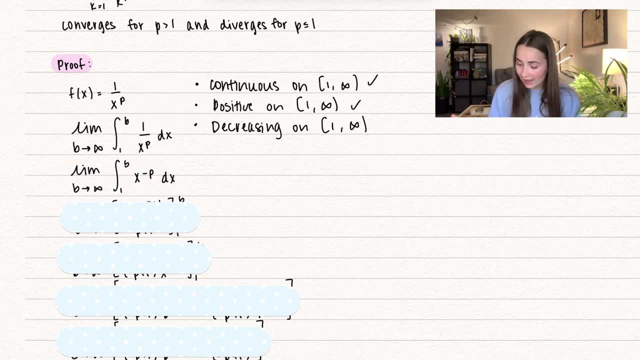 ahead and rewrite this so we can see power rule really well. I'm going to rewrite it as x to the negative p because we can go in and apply power rule. I'm going to add 1 to my exponent, so negative p plus 1, and I'm going to divide by that new exponent. But I want to go ahead and rewrite this. 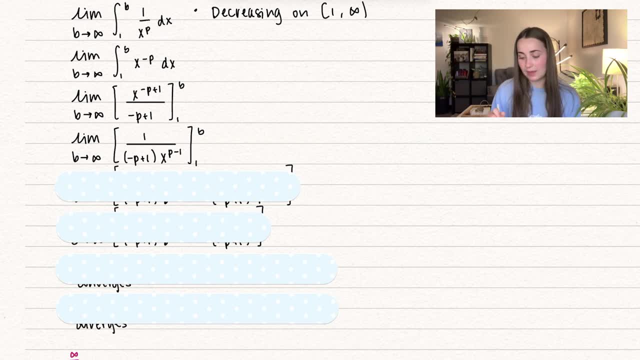 as a fraction. So what I'm going to do is I'm going to bring that x to the negative p plus 1 to the denominator. But remember that's going to flip the signs of everything. So what it becomes is 1 over negative p plus 1 times x to the positive p minus 1.. So now what? 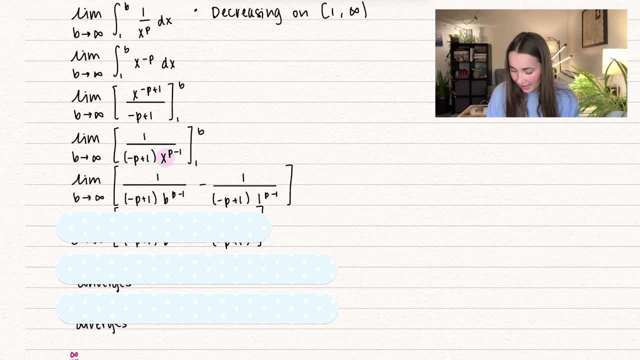 we can do is plug in upper minus lower And remember we are replacing x. So here we get our upper bound of b, Here we get our lower bound of 1, which we can actually go ahead and simplify that, because 1 to the p minus 1, that's just always going to be equal to 1.. So this right. 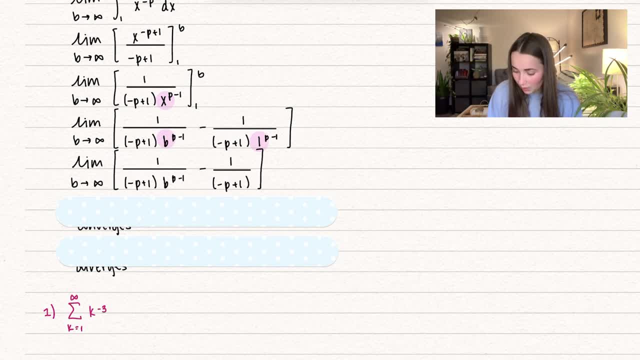 here is the limit that we're working with Now. p minus 1 here in the exponent is going to tell us a lot of information, So let's go ahead and go through it. If p is greater than 1, p minus 1 is going to be positive. So, for example, if p is equal to 2,. 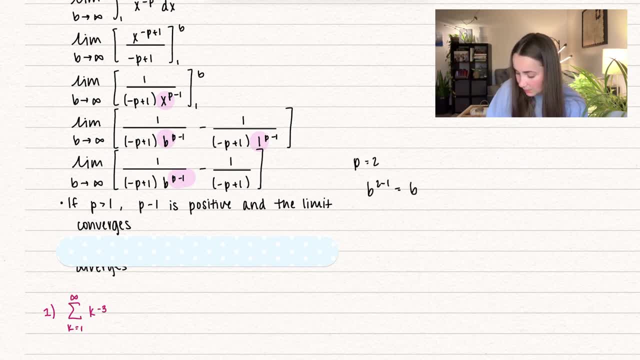 we would have b to the 2 minus 1, which is equal to b to the first. That means that the b, the infinity, stays in the denominator And 1 over infinity goes to 0. So this tells us that it's going to converge. Now what happens when p is less than or equal to 1?? If p is less than, 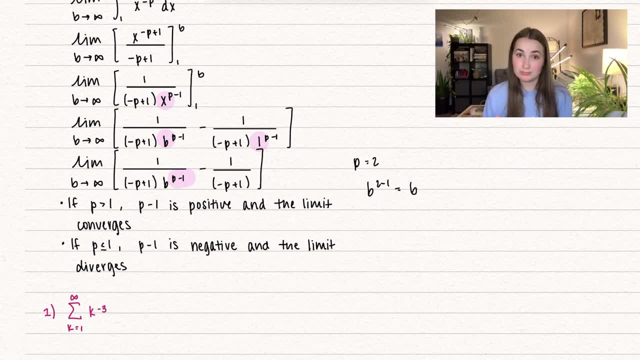 or equal to 1, or if it's equal to 1, p minus 1 is 0.. That's not going to help us. That's going to be the harmonic series, so we can ignore that for now. But if p is strictly less than 1,, 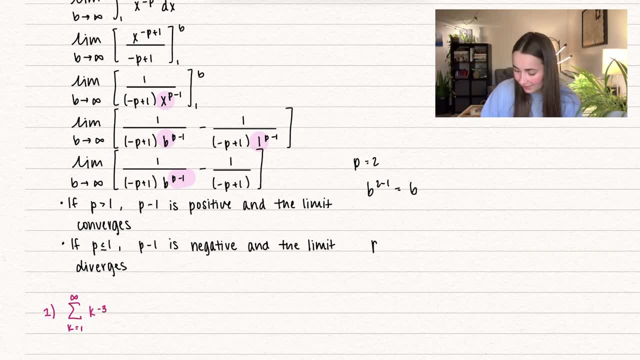 then p minus 1 is going to be negative. So what happens here is that if p is equal to 1 half, for example, we have b, 1 over b, we'll say for now, of 1 half minus 1. That is equal to 1 over. 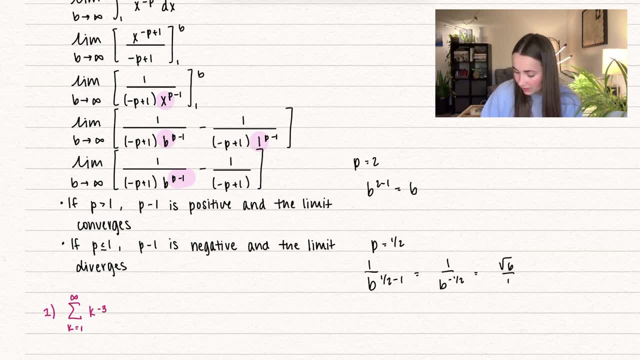 b to the negative 1 half, which actually would be the square root of b divided by 1.. So what happens is that infinity goes to the numerator And when it's in the numerator it's going to diverge. So let's go ahead and go through some examples. 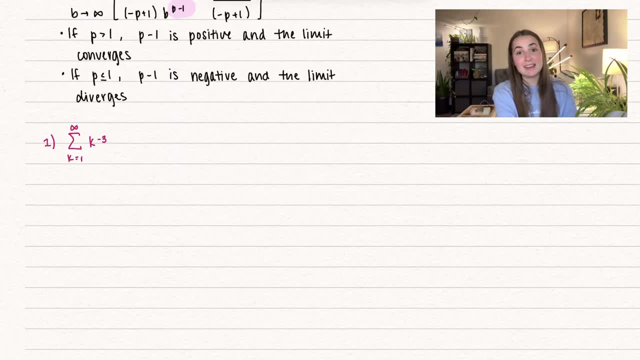 First, we have the summation: k equals 1 to infinity of k to the negative 3.. So here, what we're going to do is we're going to rewrite it so we can really see the p series going on, And I'm going to use properties of exponents and we get 1 over k. cubed p in this case is equal to 3,. 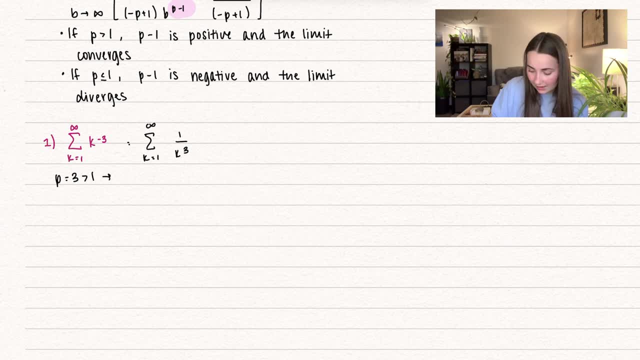 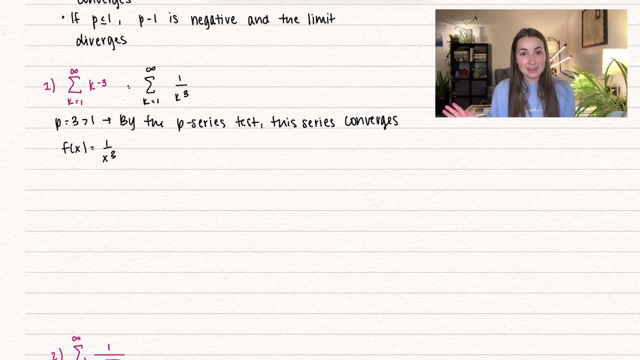 which is going to be strictly greater than 1, which tells us this series is going to converge. But let's go ahead and work it out with the integral test. We have that our function that we'll be working with is going to be 1 over x cubed. You can make sure it meets all three conditions. We know it's going to be. 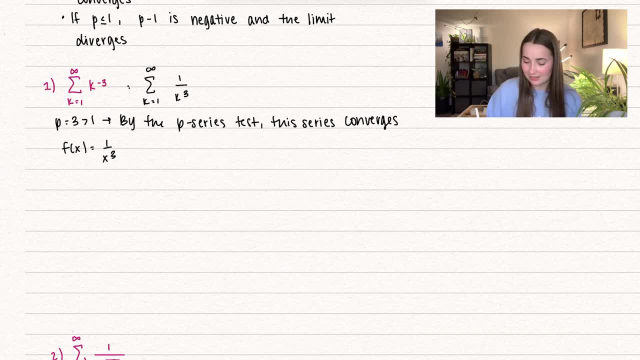 continuous. we know it's going to be positive and we know it's going to be decreasing. So here let's go ahead and set it up. The limit as b approaches infinity of 1 to b, of 1 over x, cubed dx. And I'm just doing it so we can understand the p series a bit better, And I'm 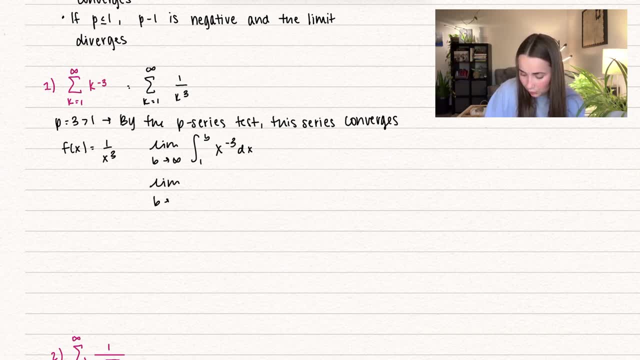 going to rewrite that as x to the negative 3, so we can really see exponent rule going on. So this becomes x to the negative 2 divided by negative 2 evaluated between 1 and b. But again, I'm going to rewrite that So that's going to be negative 1 divided by 2x squared. So here: 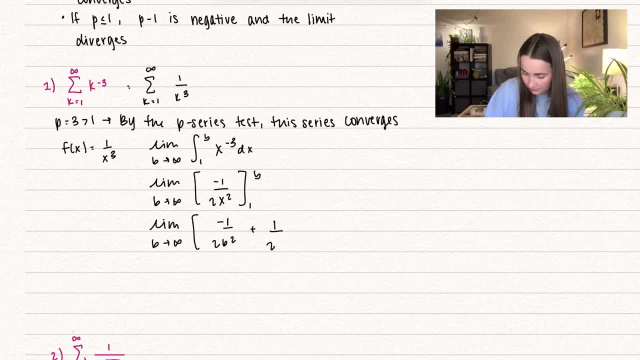 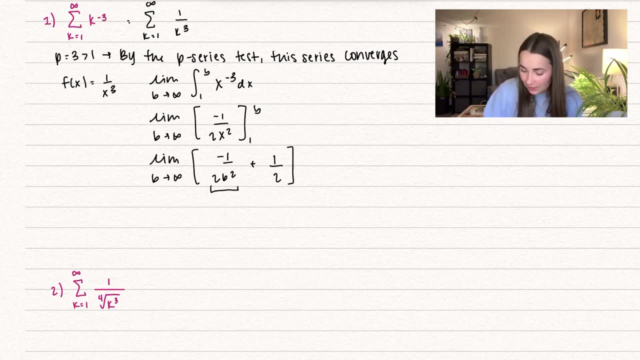 we can go ahead and plug in upper minus lower And notice what's going to happen, Since our p value was greater than 1, what happens is that this, right here, as b grows infinite, is going to approach 0. So this is equal to 0 plus 1 half, which is equal to 1 half. So also by the integral, 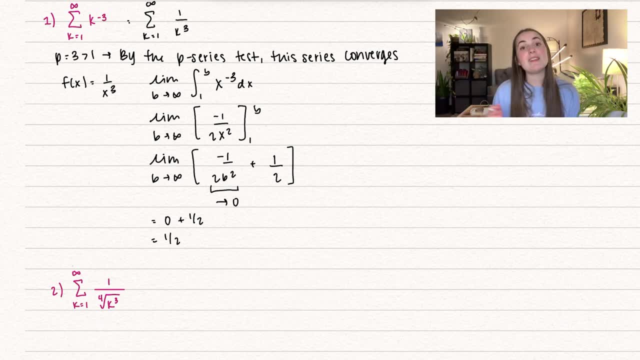 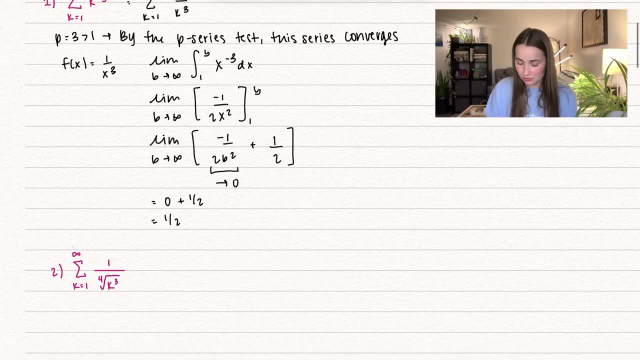 test. we can understand that when p is greater than 1, this is going to converge right. It's not going to converge to 1 half. It's going to converge to some number. It's not going to be 1 half, but it just means it's going to converge right. Let's go ahead and try this. 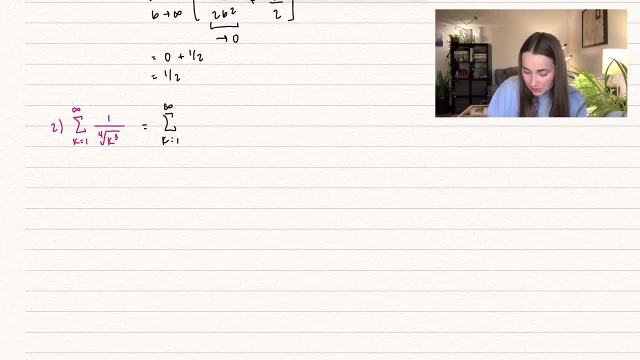 again We have the summation: k equals 1 to infinity, And I'm going to go ahead and rewrite that as k to the 3 fourths. In this case, p is equal to 3 fourths, which is going to be less. 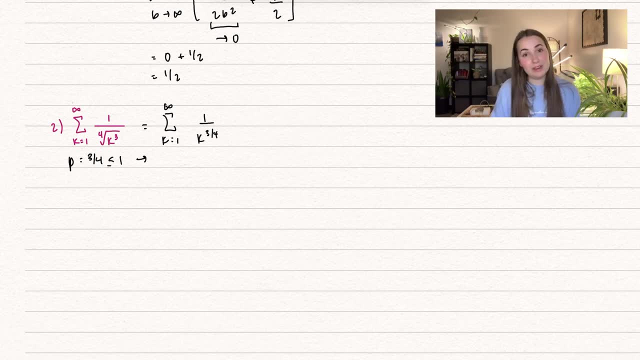 than or equal to 1, which tells us that the series is going to diverge. Let's go ahead and work it out with the integral test so we can really see what's happening. The function that we're working with is going to be 1 over x, to the power of 3 fourths. It meets all three. 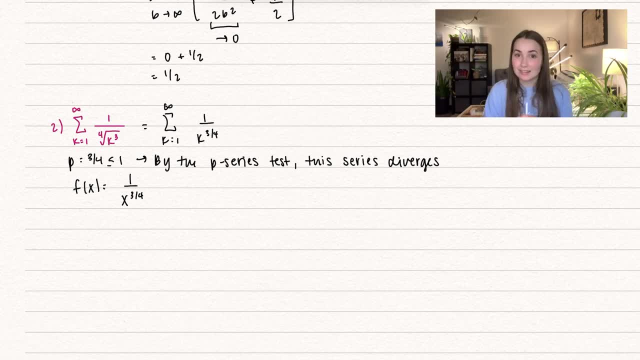 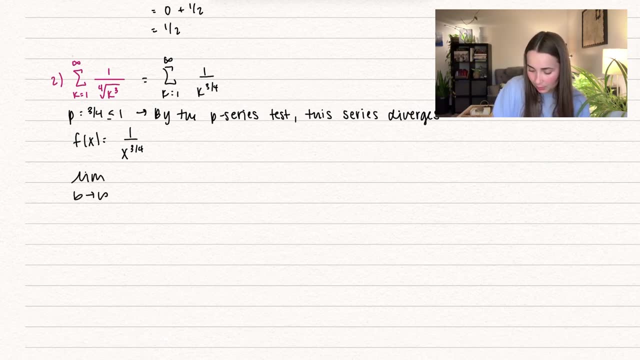 conditions. Make sure to write that down if you're taking an exam. right, It is continuous, It is positive And it's decreasing over this interval. So let's go ahead and write out our integral. the limit as b approaches infinity, We have 1 to b of 1 over x to the 3 fourths dx Again. 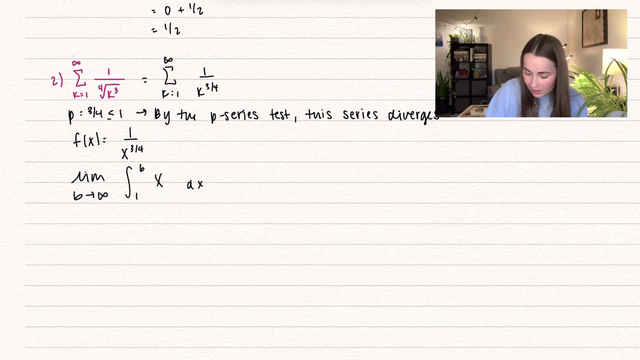 the first thing I want to do is rewrite this so I can really see power rule. So it's going to be x to the negative 3 fourths. So here we have the limit, As b approaches infinity of, we add 1 to the exponent So that becomes 1 fourth. And when we 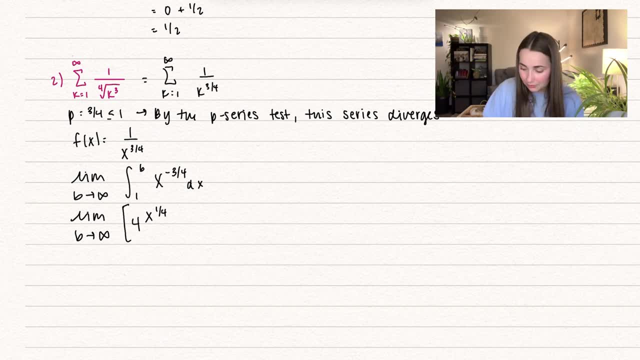 divide by 1 fourth, we can just multiply by 4. So we get 4 times x to the 1 fourth, And then this is being evaluated between 1 and b. So here I'll go ahead and plug in upper minus lower. 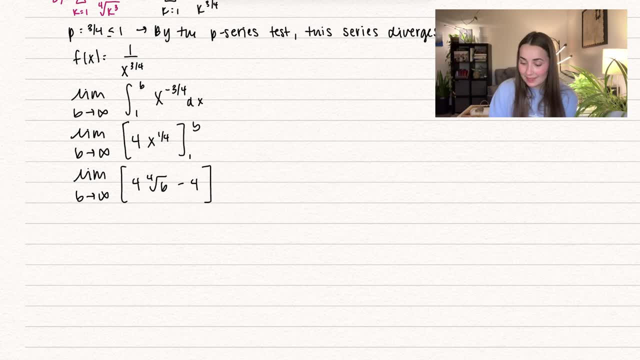 So notice here what happens when p is less than or equal to 1. This becomes infinite 4 times. the fourth root of infinity is going to go to infinity. So this is going to approach infinity, right, which tells us that it's going to diverge. So that's how the 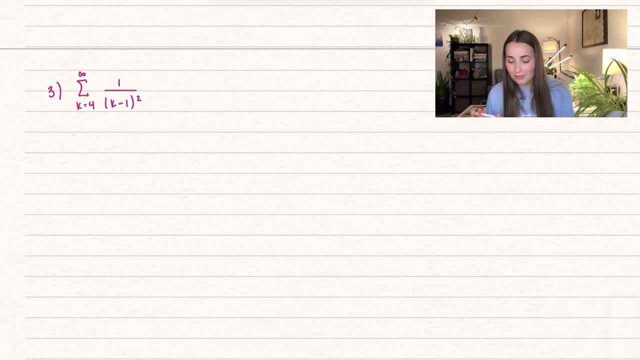 p series works out, Let's go ahead and try a bit more complicated one. We have the summation k equals 4 to infinity of 1, over k minus 1 to the power of 2.. We can manipulate this to look like a p series. So what I want to happen is I want this to be k squared right. I don't want to have 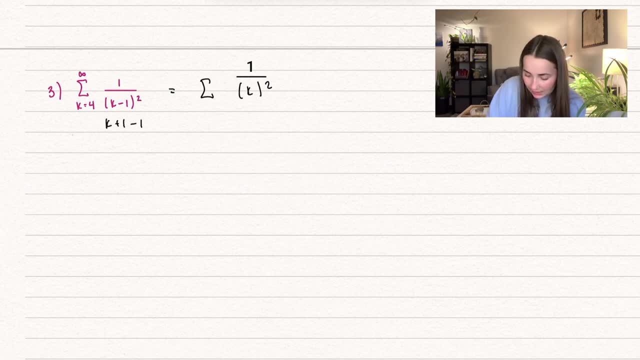 that minus 1.. So what happens is I need to add 1 to k in order for that minus 1 to cancel out. So how do I add 1 to k? Well, I subtract 1 from the index If I start at 3 instead and go to